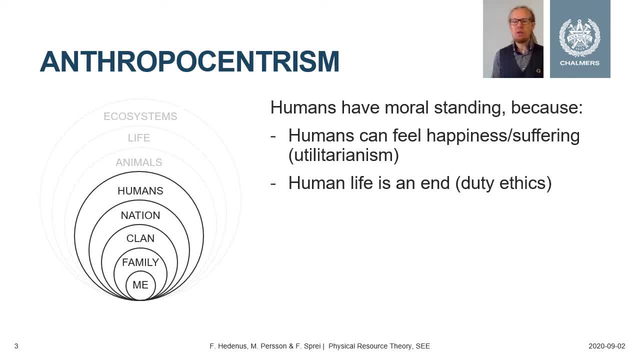 arguments for why only humans have, or why humans have, moral standing. You can base it on a utilitarian value, saying that humans can feel suffering and happiness and so on and therefore they have moral standing. Or you can base it more on a youth-ethical argument, saying that all human 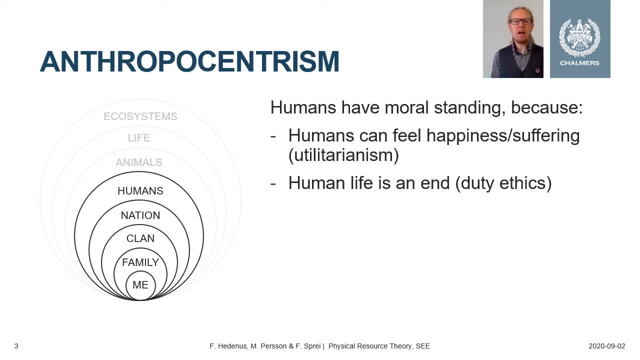 life is an end in itself, And that's a fundamental discussion. Thank you itself, and therefore all humans, have some inalienable rights. So what anthropocentrism does is that it makes a distinction between humans and the rest of nature. 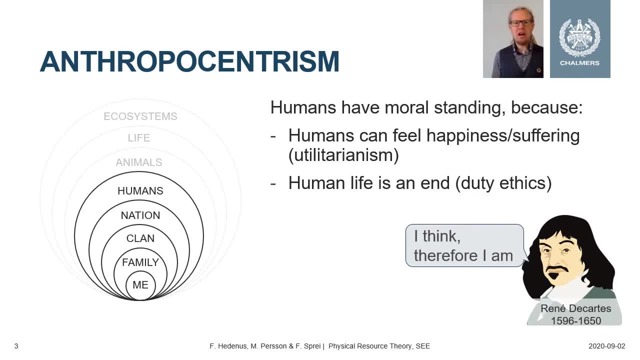 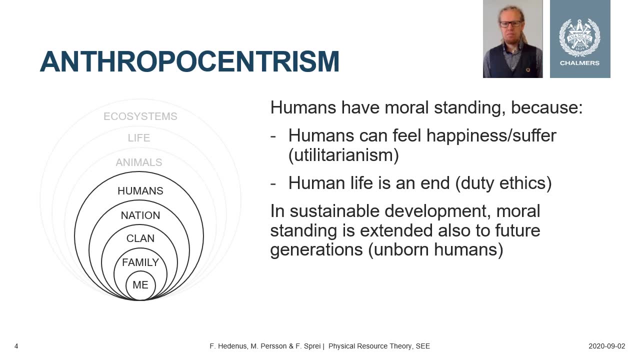 And this can be traced back to this idea of dualism, from Descartes saying his quote, I think. therefore, I am distinguishing humans from the rest of nature, So it's only humans that can have moral standing. What we do in sustainable development is that we extend moral standing from humans living. 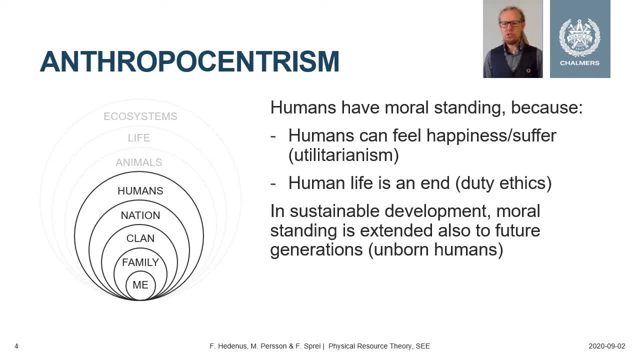 today to humans that will also exist in the future, so unborn human beings. From a philosophical perspective, this is far from straightforward, but there is quite a clear intuition here. You could argue that it shouldn't matter where on earth you are born. 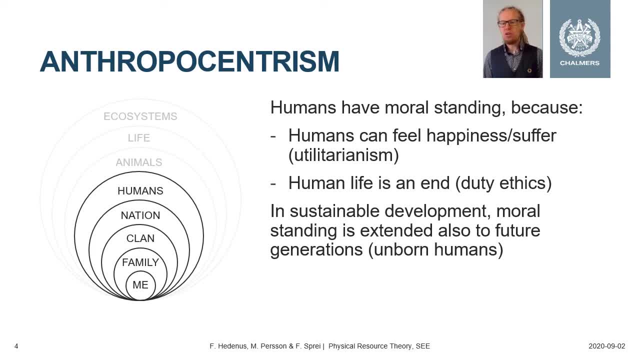 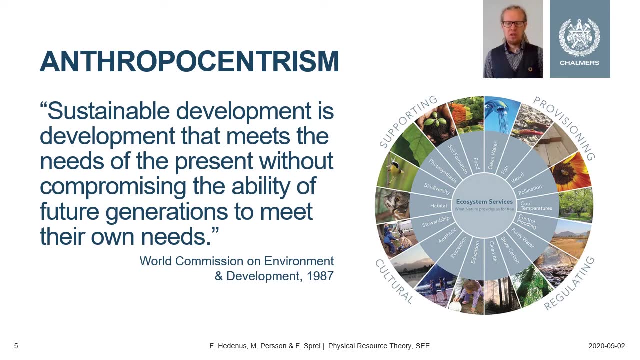 Or whether you have moral standing or not. And in the same way you can argue: it shouldn't matter when in time you are born, for whether you have moral standing or not. So the idea of sustainable development is originally an anthropocentric idea. So the standard definition of sustainable development from the Brundtland Report doesn't. 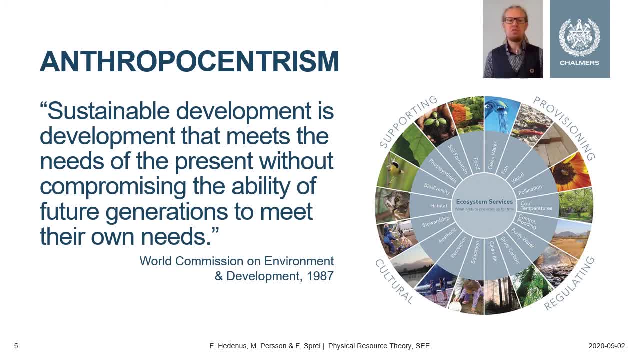 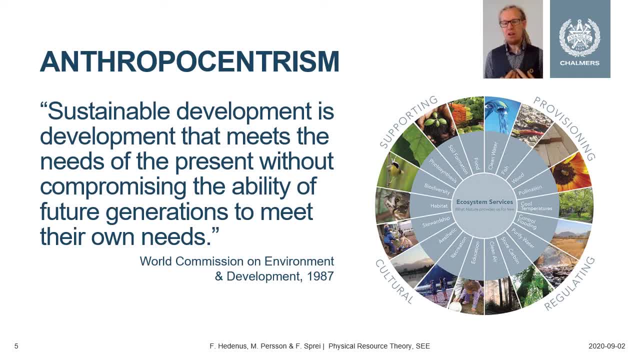 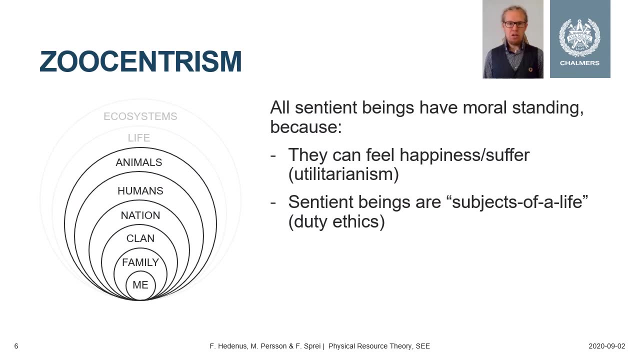 which views nature purely as an instrumental value for us humans. So nature has a value in that it provides services and benefits for us humans, not having moral standing in itself. So you can expand the circle of moral concern even further, and the first step to do that 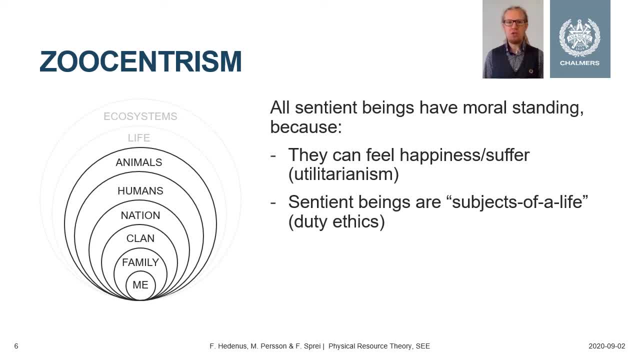 is to include. So again, that is the problem of anthropocentric heute There is a certain drive that becomes vulnerable for anthropocentrism in the scientific Calling. That being said, I'm not going todest拜拜 and talking about ent新聞. 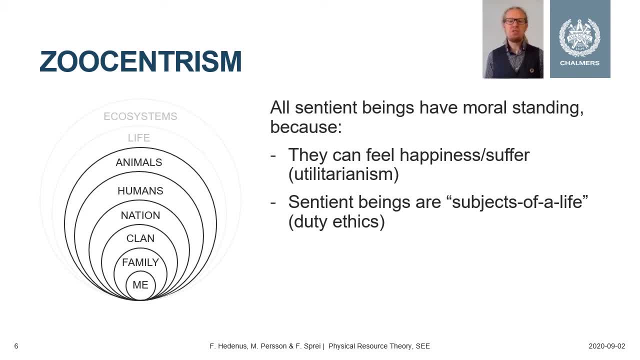 That being said, I'm not going todest freedoms. That being said, I'm not going too dej arguments, That being said, I'm not going todest- revolves around social boxing. You can go back even further if you're thinking about a sort of western philosophical tradition. 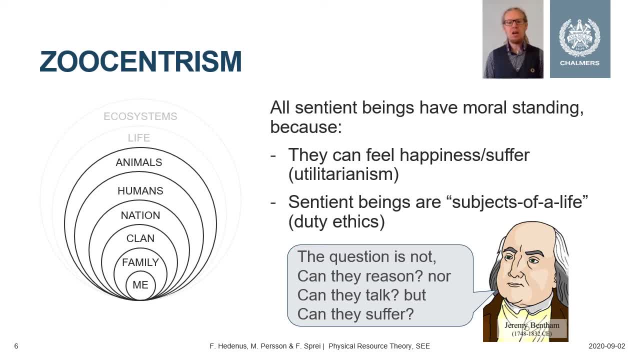 One of the first philosophers to express this idea was the father of utilitarianism, Jeremy Bentham, who said: the question is not can they reason, nor can they talk, but can they suffer? as an argument for also giving accounting for the interest of animals in utilitarianism. 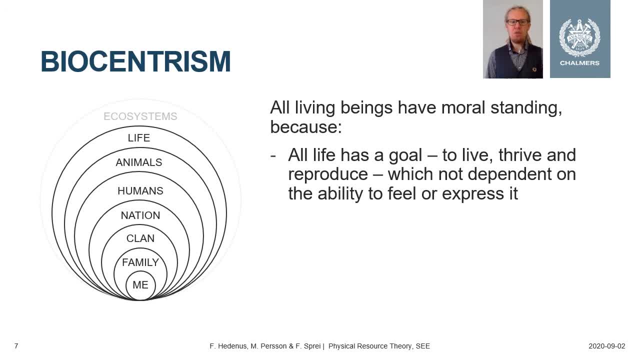 But then you can go even further. You can argue that all living beings have moral standing, So not only individual humans and animals that are conscious, but also individual plants, trees, insects and so on. This is often called biocentrism, And the argument here can be that 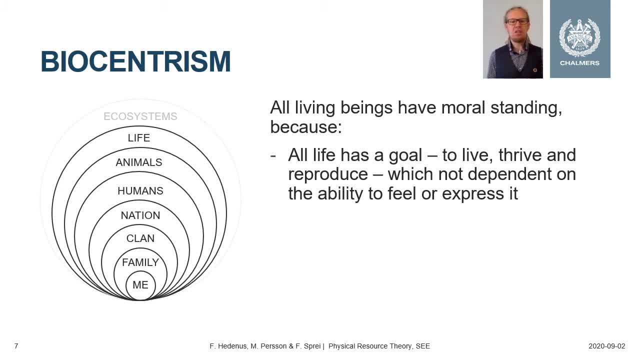 all life has a goal: to live in a certain way, to live in a certain way To live, to thrive, to reproduce. And this goal, this interest, is not dependent on whether an entity can express or feel that or not. So, therefore, all individual life should have moral standing. 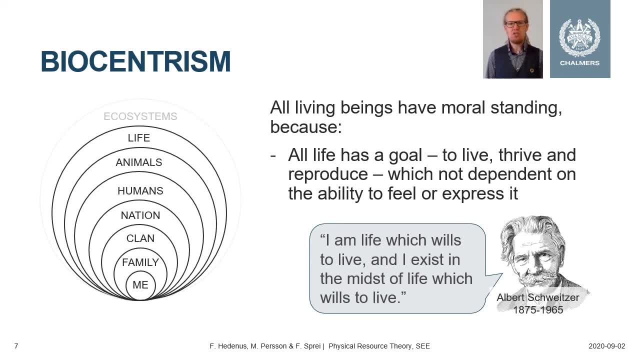 Again this. of course, this idea of biocentrism is enshrined in many sort of traditional religious beliefs, natural religions, But in the western philosophical traditions an early proponent of this view was Albert Einstein. Albert Schweitzer, who's a Nobel laureate in peace, said: I am life which wills to live, and I 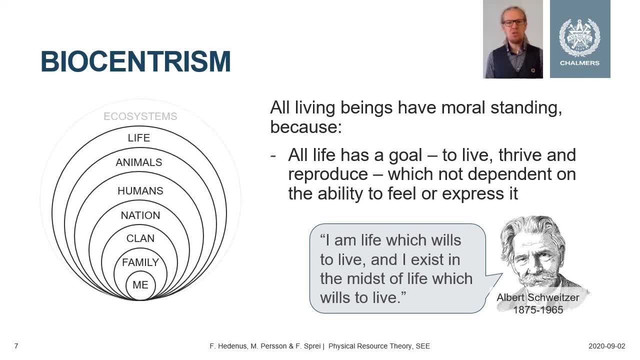 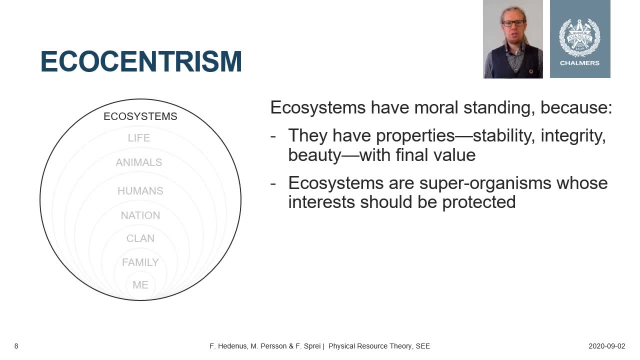 exist in the midst of a life which wills to live. Sometimes this is also expressed as reverence for life. Finally, one can expand the circle of moral concern to include whole ecosystems in what is often called ecocentrism. It's important to note there's a qualitative distinction here, So 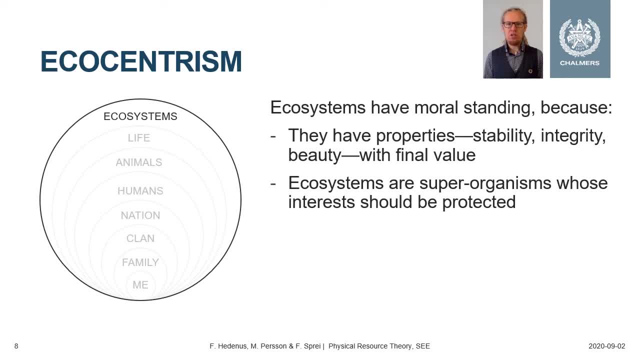 anthropocentrism, zoocentrism, biocentrism, the focus is on individual, the individual, life, the individual, human being or animal, Whereas in ecocentrism the focus is on the whole, on the ecosystem as a whole, And it's only ecosystems that have moral standing And the 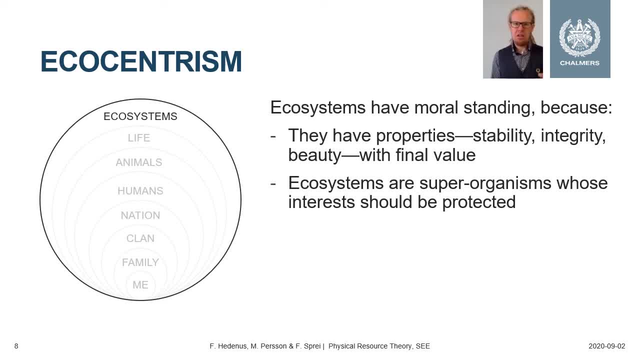 constitutions of the ecosystems. the living beings only have instrumental value, And you can argue for this based on an idea that ecosystems have certain properties: stability, integrity, beauty, which in itself has final value and should be conserved or preserved. Or you can think of 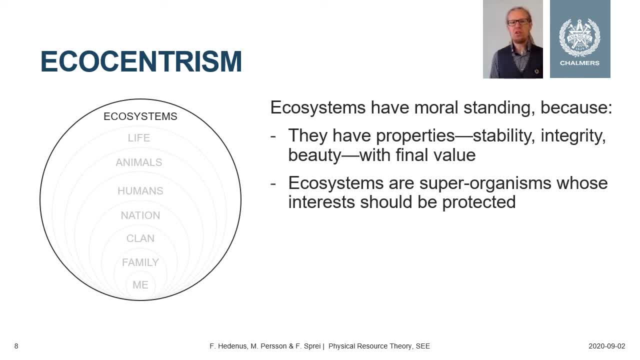 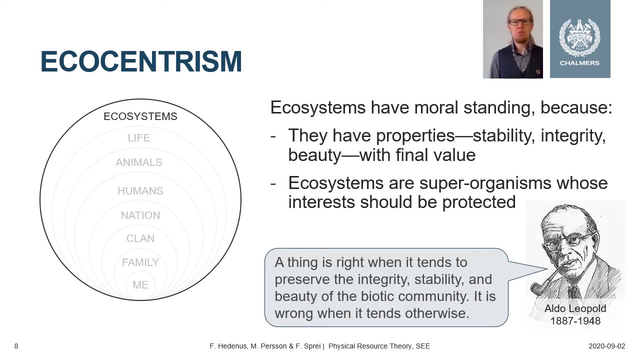 ecosystems as superorganisms- You might have heard of the concept of Gaia- And the interest of these superorganisms should be accounted for when we decide what is right and wrong to do. Again, in the Western philosophical tradition, one of the first people to sort of promote this idea with some impact was Aldo Leopold. 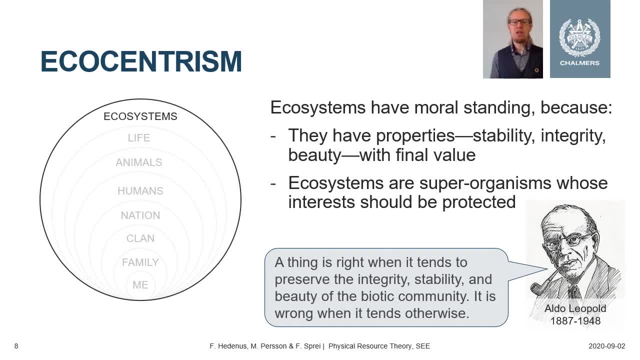 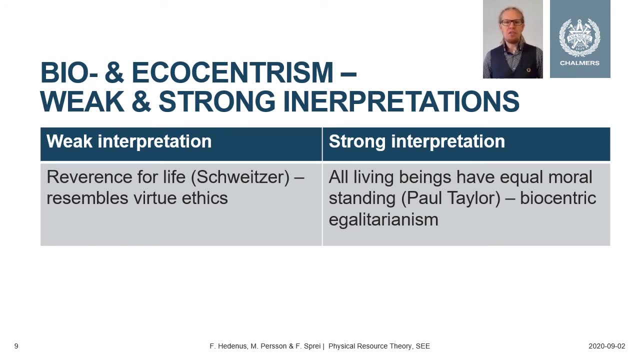 a US conservationist who said: the thing is right when it tends to preserve the integrity, stability and beauty of the biotic community. It is wrong when it tends otherwise. So it should be noted that, while moral philosophy have dealt extensively with anthropocentrism and 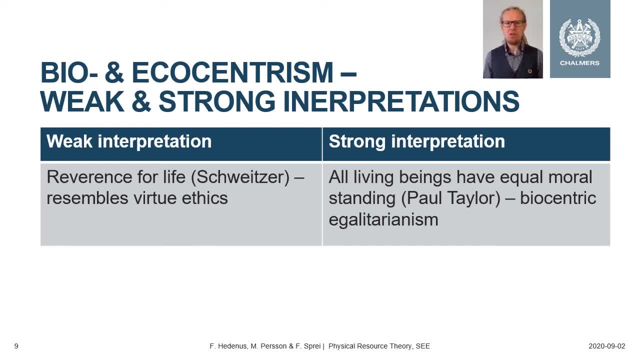 deciding on what's right and what's wrong. it's not always the case, And so I think that's a key issue here, And it's important to highlight that the concept of biocentrism and eco-centrism has been much less explored And almost in relation to bio-centrism, which is the idea of 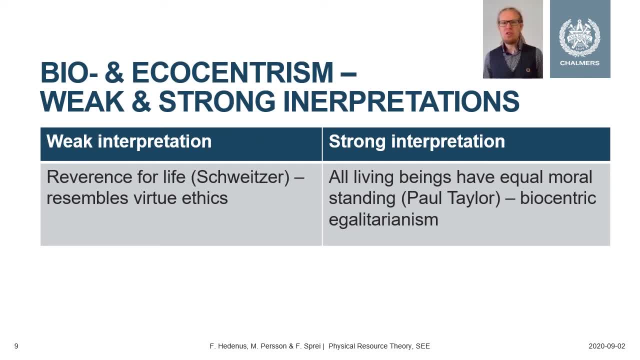 the human rights and including the animal and utilitarian thinking. the concepts of bio-centrism and eco-centrism has been much less explored. So if we take Albert Schweitzer's idea of bio-centrism, it's quite vague and fluffy. It can more be viewed as some 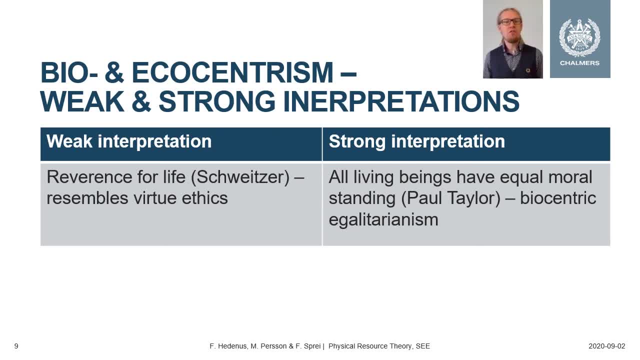 sort of virtue ethics. we should have reverence for life, try to tread as lightly as possible, try to do things that are not just about human rights and ethical values, but rather about the human rights. So the concept of biocentrism and eco-centrism has been much less explored. 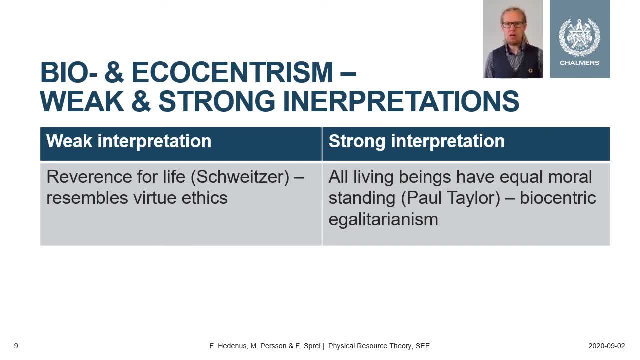 life, try to tread as lightly as possible on earth, avoid hurting other living beings. but it doesn't really detail what to do when, when human interests conflict with other, with the interests of other living beings. so one of the few philosophers to actually try to develop a more stringent 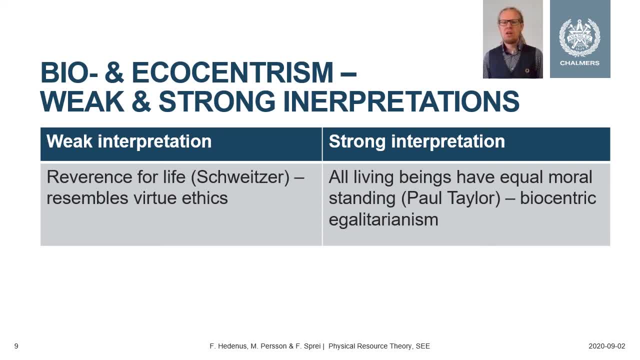 theory around biocentrism is paul taylor who's, who argues that that all living beings have equal moral standing, something you can call biocentric egalitarianism, which is a stronger interpretation of of biocentrism. of course, what this means is. it doesn't mean that that humans or 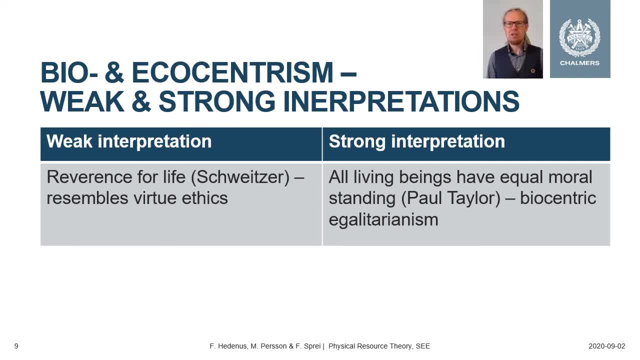 other human, other living beings can never hurt another living beings. we have the right to to fulfill our basic needs. so we, if we need to hunt or if we need to kill other plants in order to live, that are right for us to do, in the same way that the lion is not wrong when it kills its prey. 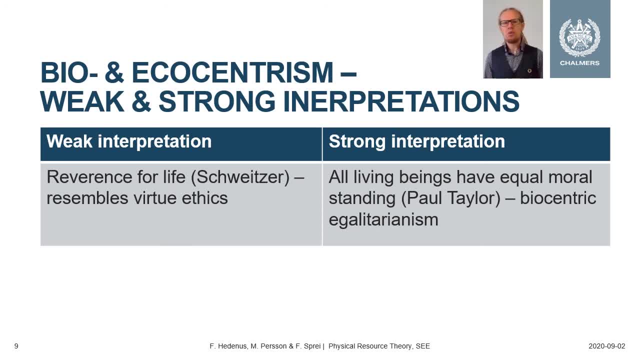 the question is, of course: how far do you extend? what do you include in in these basic human needs? and here paul taylor does go a bit further and say: well, we also have needs to develop ourselves as individuals or develop our civilization. so if we need to, 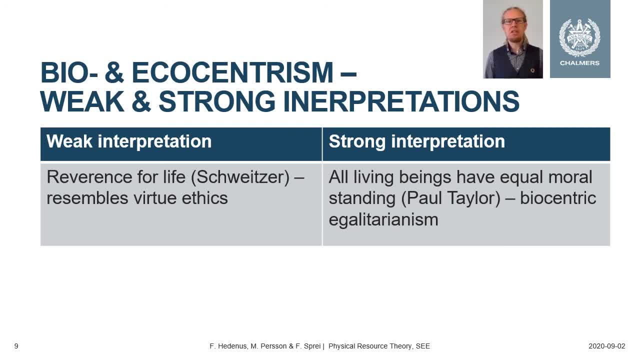 cut down a forest in order to build a library. that can also be moral, morally permissible and in that way. that way you could say that he goes a bit more towards the weaker interpretation and saying that human interests do take preference over the interest of some other living beings. 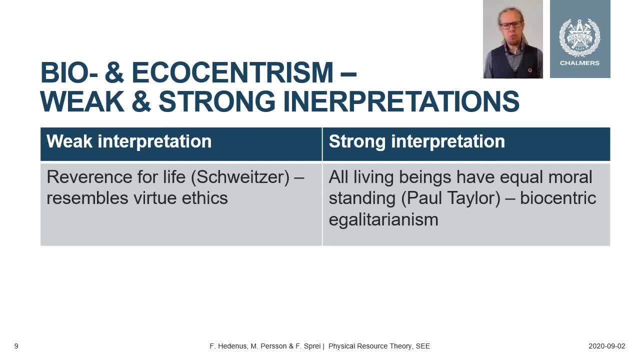 But so you can view biocentrism in a stronger or weaker sense and in the same way with ecocentrism. So in a strong interpretation of ecocentrism argues that only ecosystems have moral standing, They are the only entities, And individual beings have only. 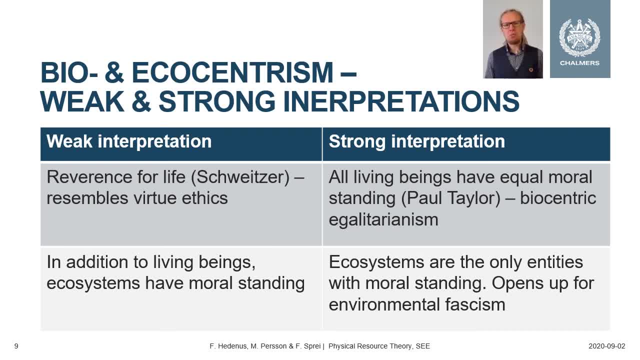 instrumental value, And this opens up to what can be called ecofascism, So setting aside human rights for the rights of ecosystems. So it can be a right to hurt or even kill human beings if that is what is best for the ecosystems. On the other side, a more weak, interpretation of ecocentrism is the idea that human rights are the only things that matter. So it can be a right to hurt or even kill human beings if that is what is best for the ecosystems. So it can be a right to hurt or even kill human beings if that is what is best for the ecosystems.